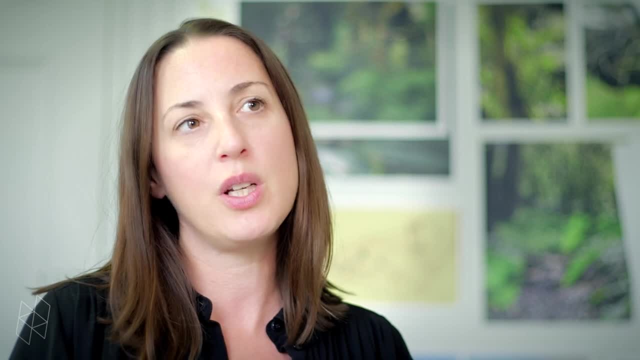 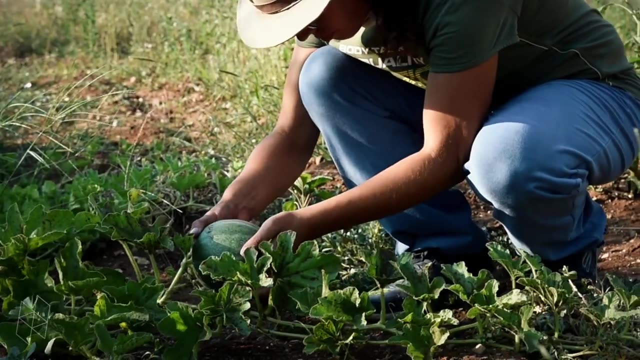 we're in a very unique role because we can work directly with the community. we can serve in stewardship and advocacy for the land itself and for those that have a close kinship with it. Sea level rise will be felt, I think painfully, in certain cities first. Miami is among those first. 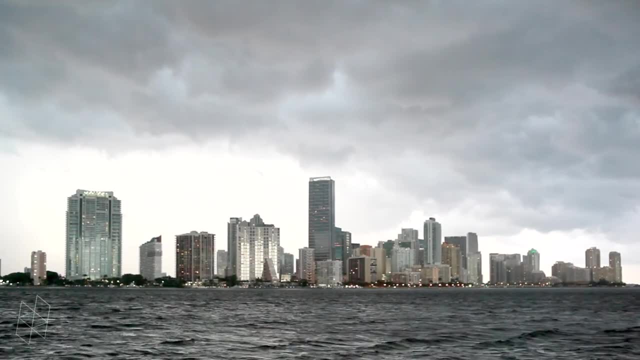 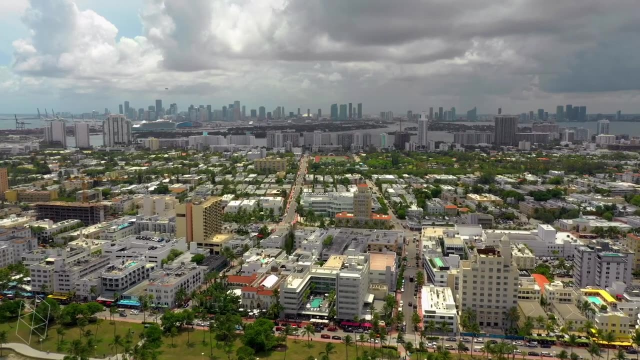 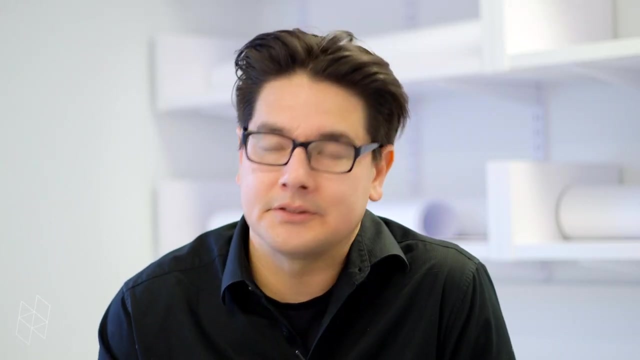 partly because of its location, partly because of its elevation, partly because of its building boom and the kind of relentless and speculation. I'm teaching a studio on the topic of climate change and Miami. Even though it's a kind of an architectural studio, it does touch on. 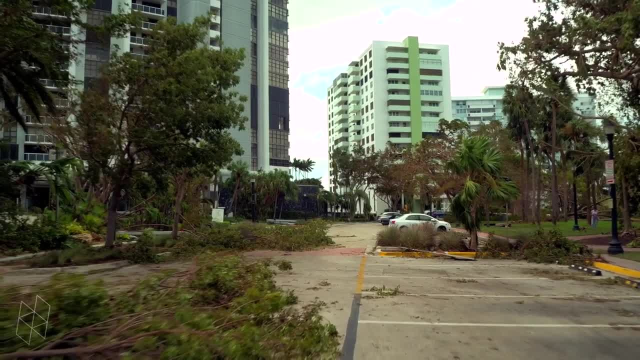 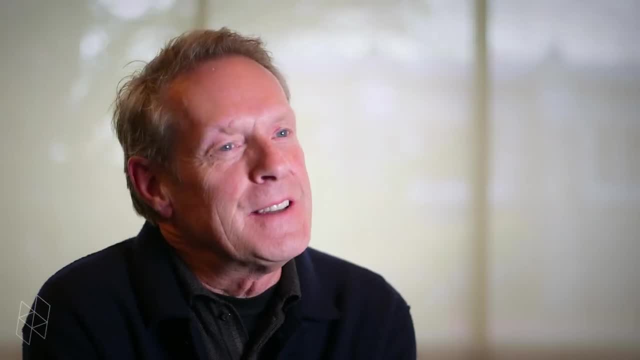 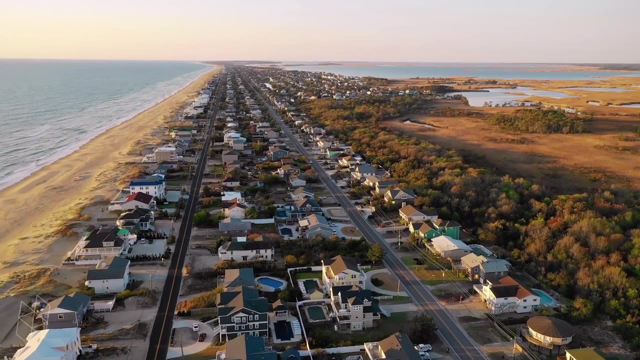 issues of urban design and social justice politics, climate justice, climate gentrification. My current studio is entitled Adrift and Indeterminate: Designing for Perpetual Migration. on Virginia's Eastern Shore, We know that the land is subsiding and that the sea level is rising and that the weather is 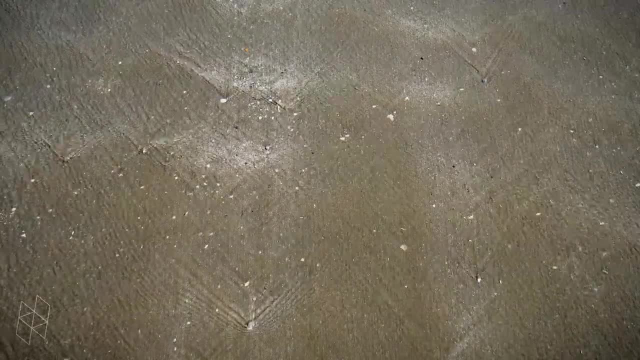 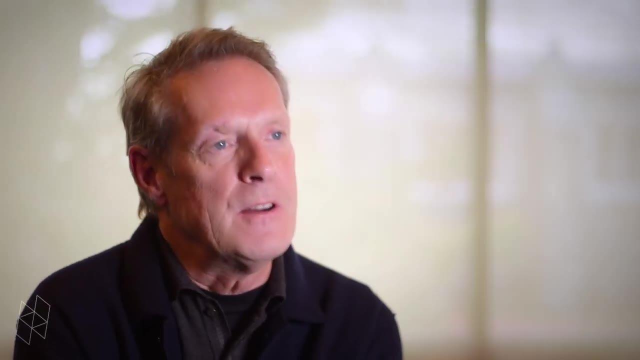 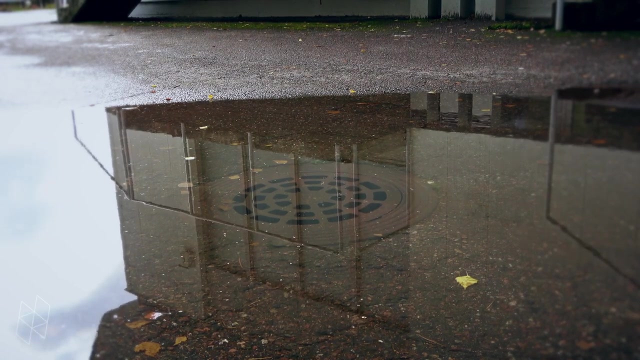 more turbulent and that surges are happening with greater frequency. The people that we spoke with think of it as erosion and we speak in practical terms about it, and so the students have really taken this to heart and they're tackling things that people face every day as design problem. We're working with things. 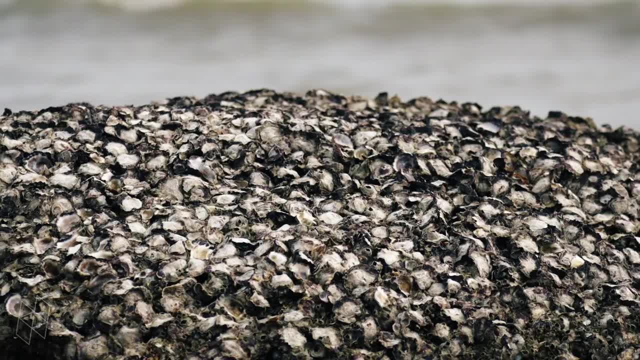 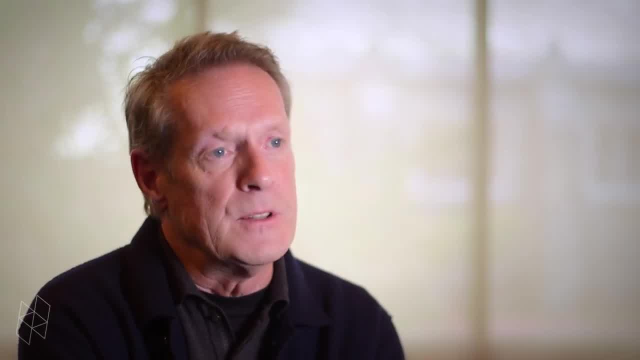 like protection. They're building oyster reefs and this is part of what we think of as land protection strategy. They have been migrating upland and this is another thing that we're designing- Designing to move up and in. We're looking at how salt intrusion into. 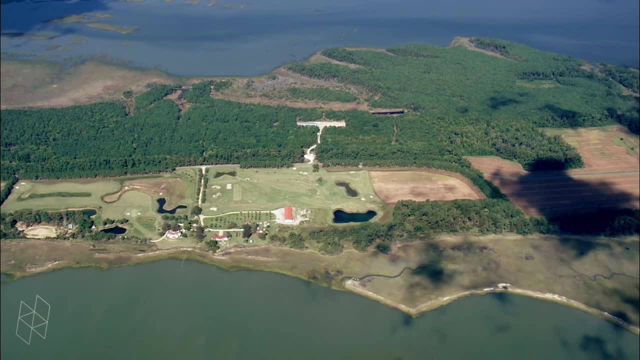 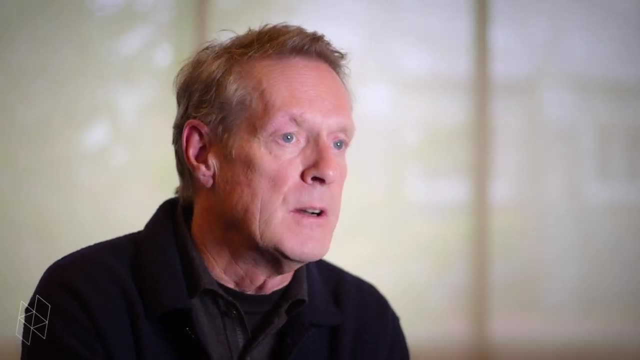 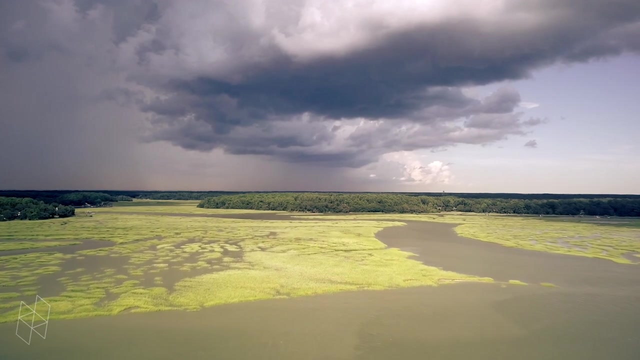 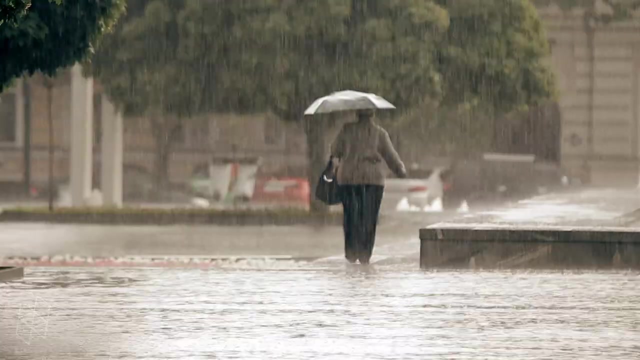 the farm soils are causing a migration of the farming itself, and we're seeing that aquaculture is beginning to replace farming in some places where we now have essentially protected grasslands that are submerged. We need land-based practices that are closer to place and not models that are global in scale and in scope. That is one. 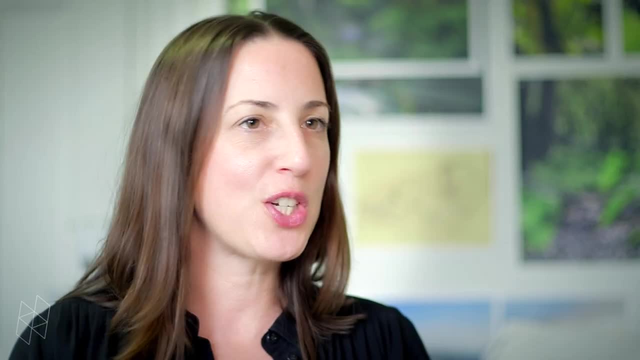 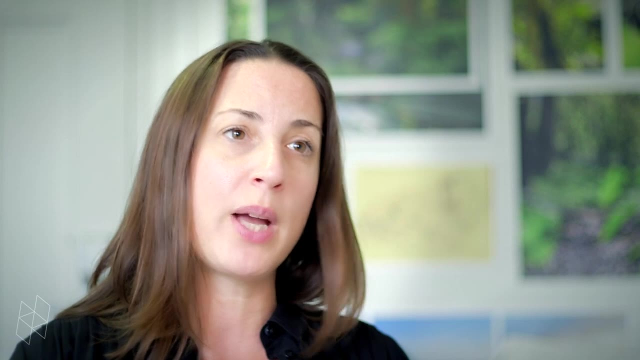 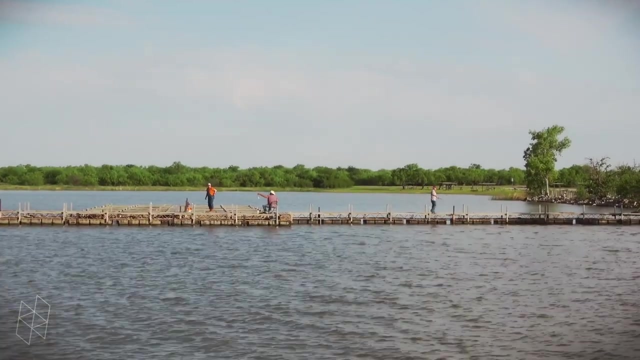 of the tricks of our trade that plays into globalization and capitalism that in fact, feeds the climate dislocation itself. How can we act in adaptable ways to these negative effects? And that's what design can really do is bring optimism to a community and work with governance to unpack and unravel some of the standards that we're stuck in. Subtitles by the Amaraorg community.